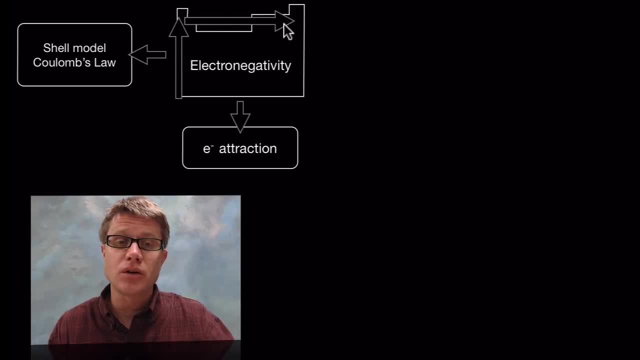 to the protons that are found in the nucleus, And then, as we move over to the right, those positive values are going to increase And we're also going to increase that attractive value. And so, based on those electronegativities, 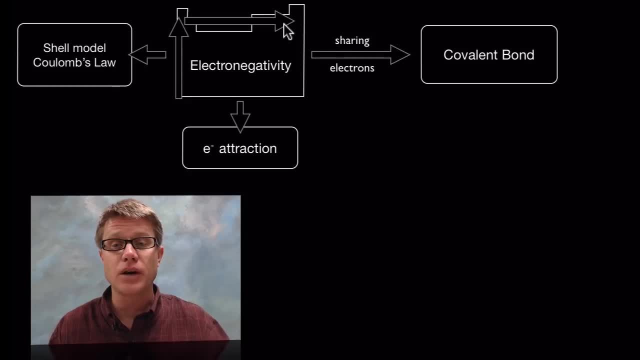 we can look at the atoms inside a molecule and we can figure out: is it a covalent bond? And if so, what type of covalent bond is it? Now, if those electronegativities are exactly the same, then we call that a nonpolar covalent bond. An example would be oxygen. that you're 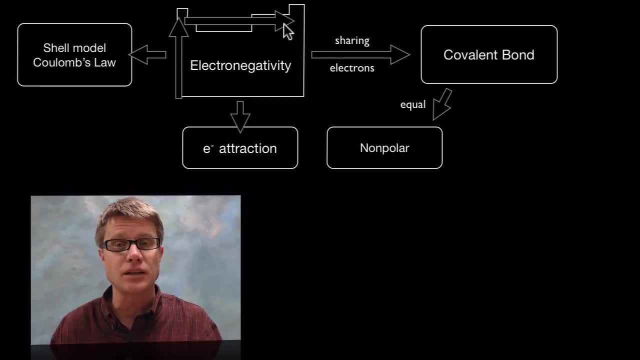 breathing right now. It's two oxygen atoms. They have the same electronegativity, So they're going to share the electrons equally. Also, you should know this- If it's a carbon and a hydrogen that are attached together, carbon is really good at sharing its electrons and 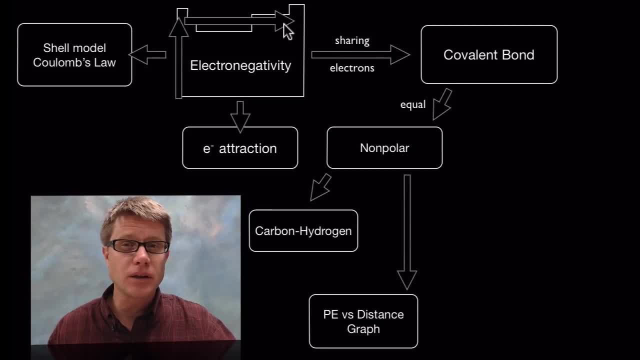 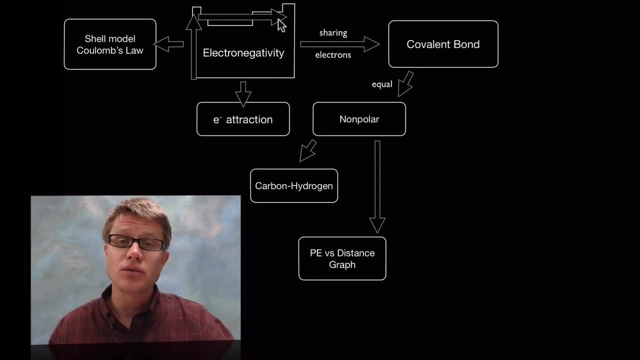 so we generally call that a nonpolar covalent bond. We can look at these bonds using a graph, where we graph the potential energy on one side and then the distance between the atoms on the other side, And so what becomes apparent is going to be the bond length, how far those 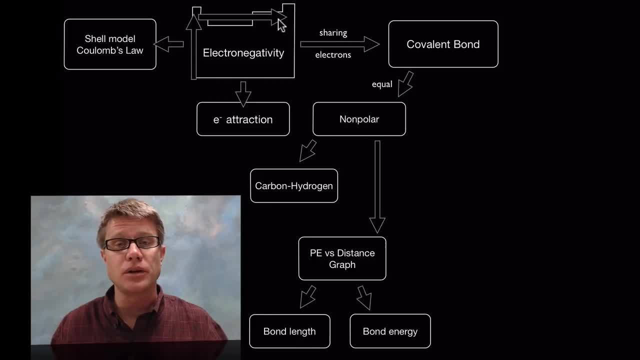 atoms are apart, and then the bond energy. How much energy would we have to put in to break those atoms apart? Now, if the electronegativity is different, then we call that a polar covalent bond. And so when we do that, we have something called a dipole, where there's a partial positive 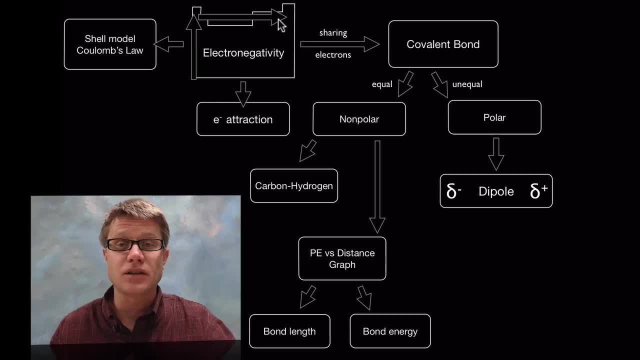 and a partial negative charge. Whichever one has the highest electronegativity is going to have that negative charge. But even though we may have differences in charge, we still have conservation of charge over that whole molecule itself. Also, as we move from covalent 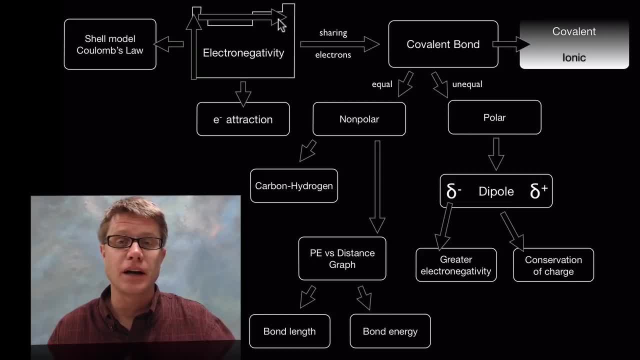 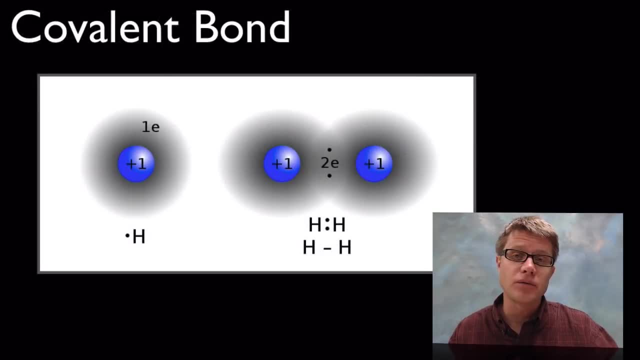 bond to more and more electronegativity, we start to move into what are called ionic bonds, And it's a gradient, It's a continuum, And so we can measure these to tell the difference between them. And so a covalent bond, remember, is going to be sharing of the electrons. So 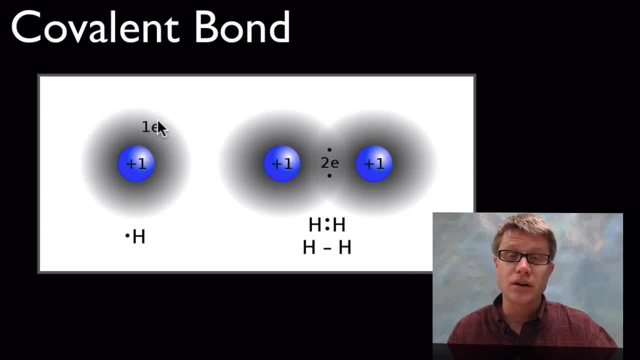 a great example would be hydrogen, hydrogen, hydrogen and hydrogen, And then we can measure hydrogen gas. Hydrogen has one electron in its outer shell. It would like to have two, And so it can share that one electron with another, hydrogen atom, And now we have the. 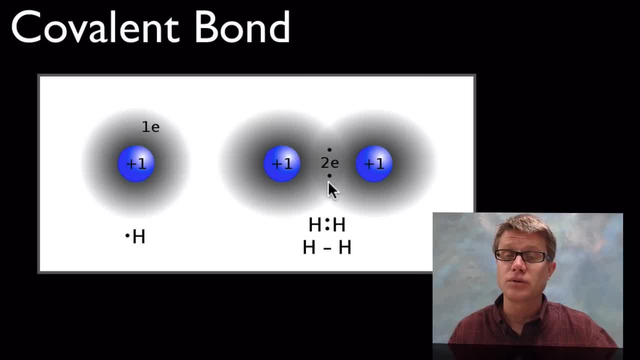 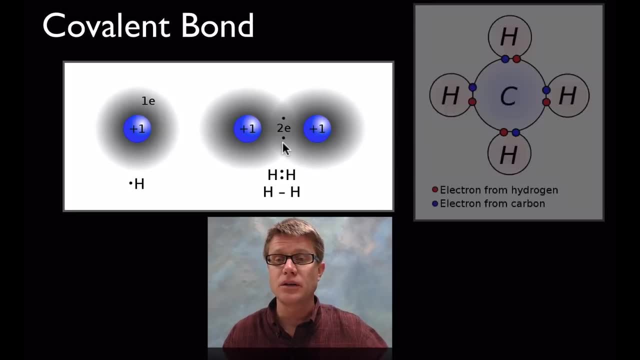 sharing of these two electrons, And so we have a covalent bond between the two. Carbon, for example, has four valence electrons According to the octet rule. it would like to have eight, And so what it can do is it can share each of those four electrons with another hydrogen. 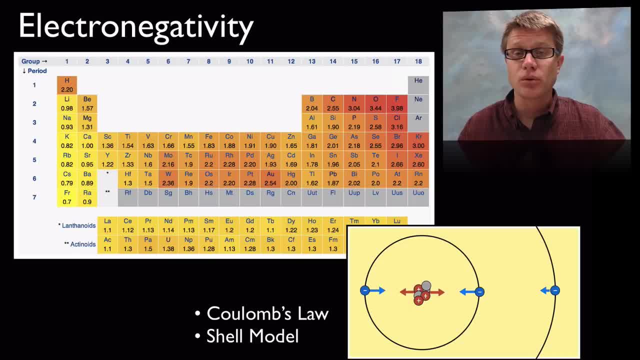 atom, And now we have methane, which is going to be a non-polar covalent bond, And so here's that. electronegativity, Remember, as we go up on the periodic table, it's going to increase, And then, as we go across, it's going to increase as well. Now, why is it increasing when we 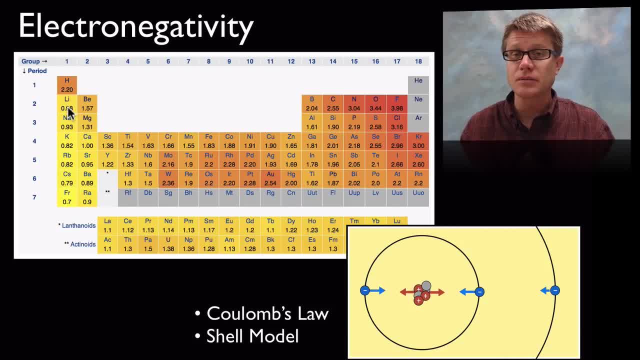 go up, It's because the atoms are becoming smaller. And as the atoms become smaller, those electrons are closer to the nucleus, and so there's going to be a greater charge. And as we move across, you can see, the electronegativity is increasing as well, because we're increasing. 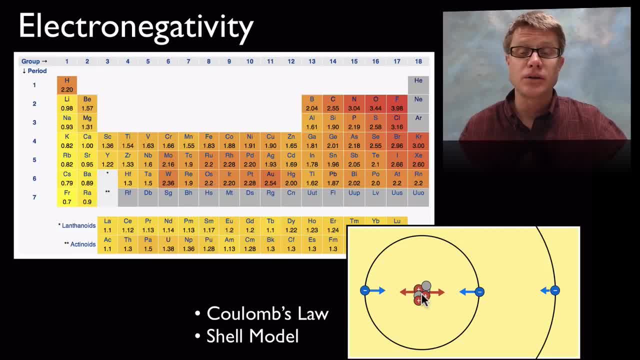 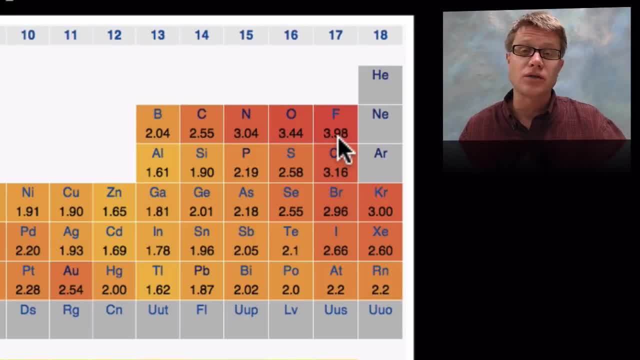 the amount of positive charges on the inside, And so we're increasing that pull. And so you can see that fluorine is going to have a higher charge, And so we're going to have the highest electronegativity on the periodic table. That means it wants electrons more. 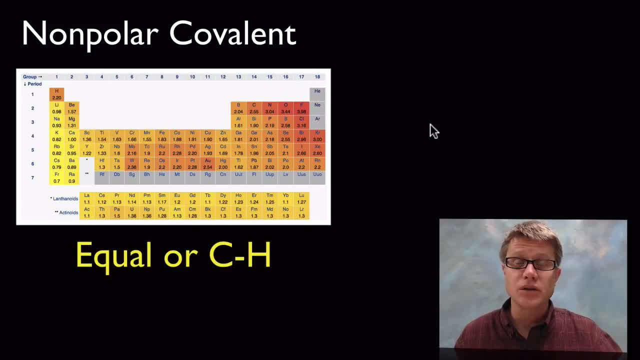 than any other atom. And so if we have two atoms that are sharing electrons and the electronegativity differences are zero, we call that non-polar, So oxygen, for example. If we look at oxygen, its electronegativity is 3.44.. So if we compare it to itself, it's going to be no difference. 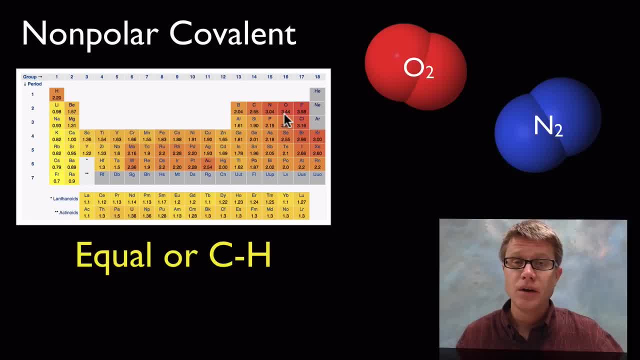 between the two, So that would be a non-polar bond. Same thing with nitrogen. Remember: if you have hydrogen, they're going to share the electrons equally, And so we'd also call that a non-polar covalent bond, like in methane. Now we can study these using a graph like: 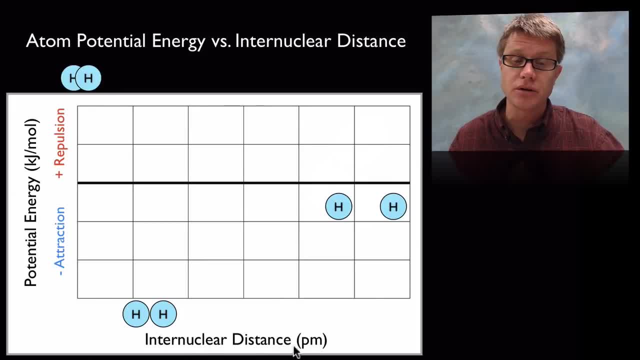 this where we put potential energy on one side and then we put inner nuclear distance between the two. So let's start with hydrogen or H2. If we have two hydrogen atoms together, as we move them really close together, they're going to want to push on each other In other. 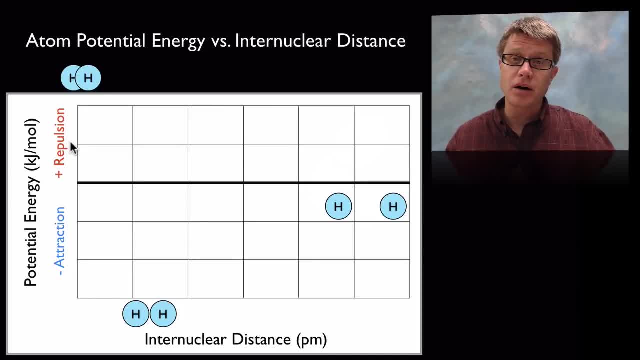 words. there's going to be repulsion As we move them farther apart. eventually they're going to get into an area where there's this sweet spot between attraction and energy. So as we move them really close together, they're going to want to push on each other In other 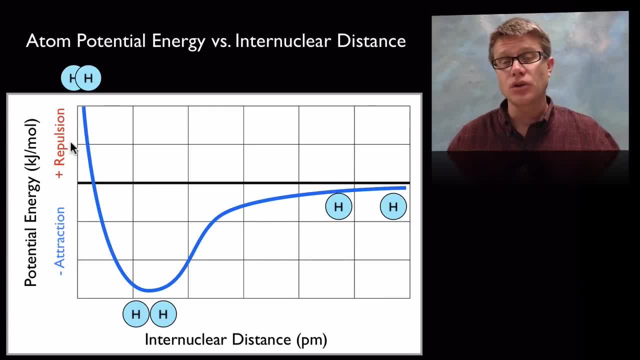 words, there's going to be repulsion, And then, as we move them really far apart, they're going to be so far apart that Coulomb's law says there's not going to be a great enough force to pull them together. And so if we're below this line, it's attraction. But what? 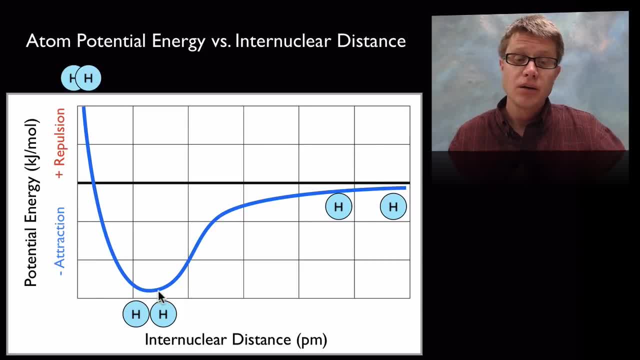 we'll find is when we have the perfect distance apart we're going to reach. what is the bond energy and the bond length of those two atoms. In other words, bond length is going to be how far generally hydrogen atoms are going to stay apart And bond energy is how much. 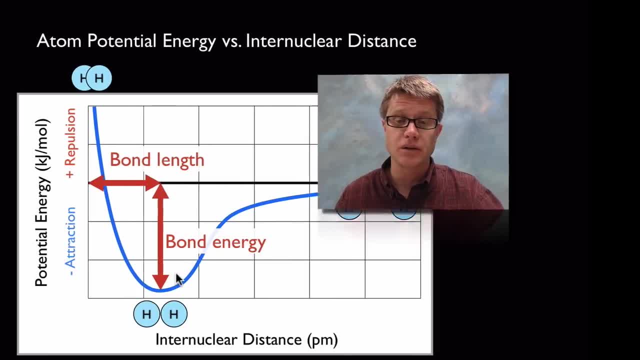 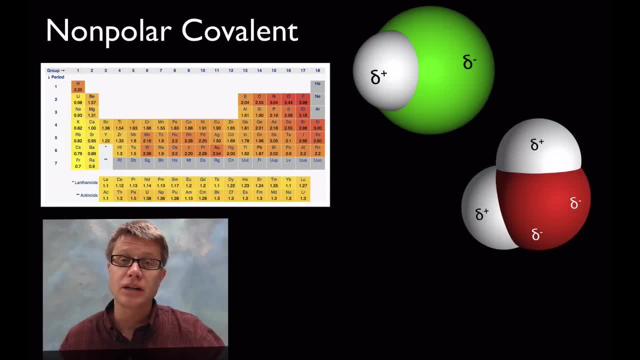 energy would we have to put in to actually break that hydrogen apart, And so this graph is incredibly important. When we're looking at nonpolar covalent bonds, what we're going to find is that their electronegativities are different, So this right here would be: 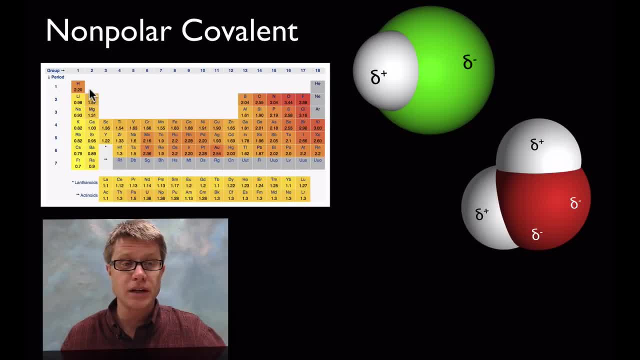 hydrochloric acid. If we look at chlorine 3.16 and hydrogen 2.20, there's a difference between those electronegativities, And so the chlorine is actually going to be a negative charge and the hydrogen is going to have a positive partial charge. Or if we look at 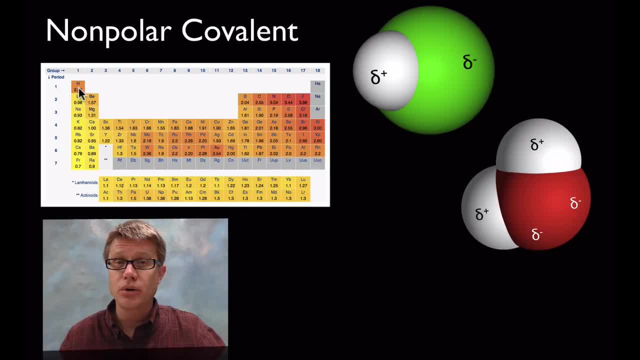 water oxygen at 3.44.. Hydrogen at 2.20.. Hydrogen at 2.40.. Hydrogen at 2.50.. Hydrogen at 2.20. zero, And so the oxygen is going to pull those electrons closer to it. So you're going to 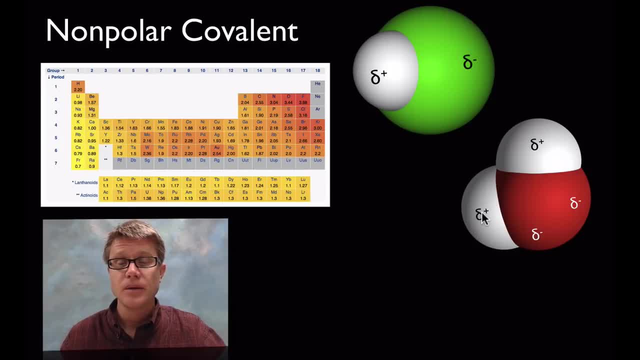 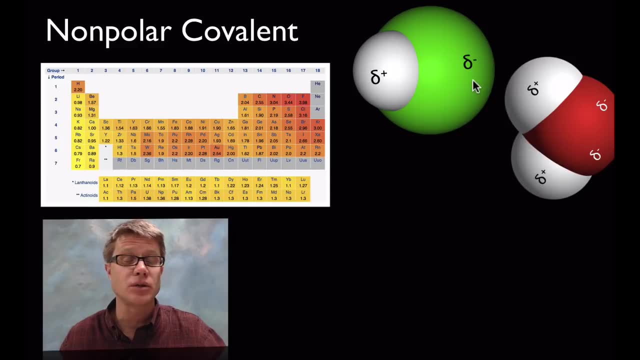 have a partial negative charge here and then a positive charge out here, And that really allows us to have water attracting the hydrochloric acid. There's going to be a dipolar charge, and the connection between those two would be intermolecular at this point. And so how? 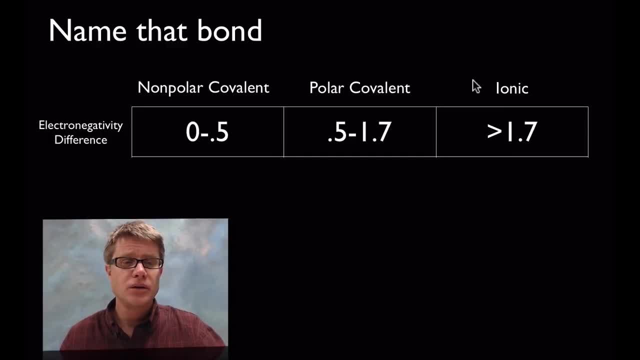 do you figure out what type of bond it is? Well, there's one quick way to do it: You could just look at their electronegativity differences on that chart. And if it's less than 0.5, it's generally going to be non-polar. If it's between 0.5 and 1.7, it's going to be polar. 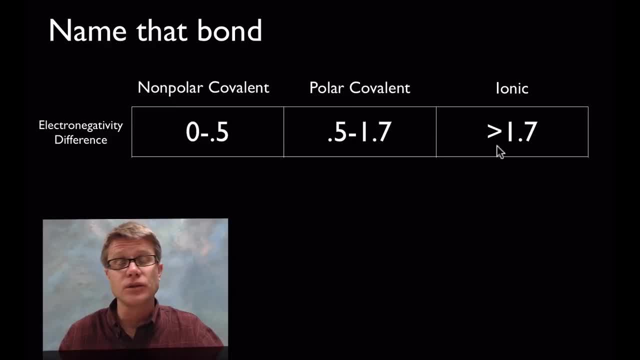 covalent And if it's greater than that, generally it's going to be ionic, And we'll talk about that in the next video. That's not a great way to do it. Better ways are to look at what's being connected. Generally in covalent bonds it's going to be two nonmetals. In ionic it's. 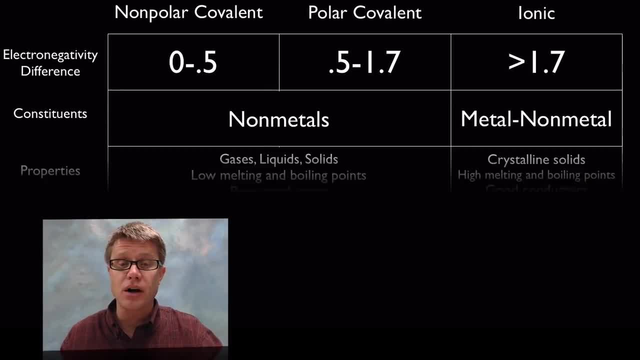 going to be metal and nonmetal And then, more important than that, we should look at the properties, And so, if we're looking at covalent bonds generally, we're going to have gases, liquids, solids, Low melting and boiling point and they're going to be poor conductors And 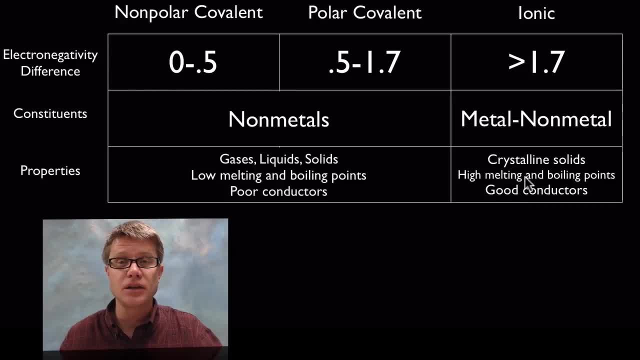 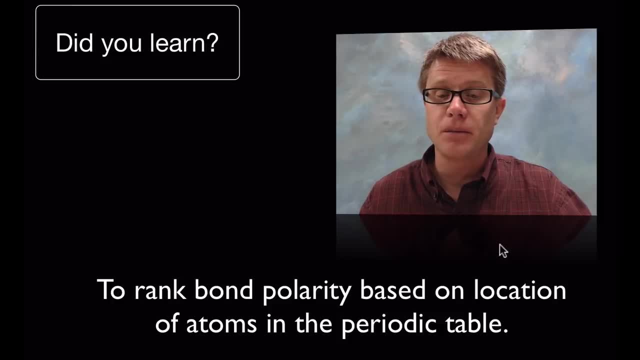 so, as we move to ionic, it's going to be a crystalline, solid, high melting boiling points and we're going to be good conductors, especially when we dissolve them in water. And so did you learn the following: to rank polarity based on location of atoms in the periodic table. 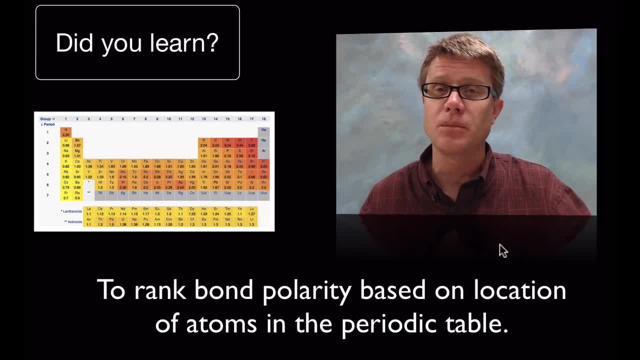 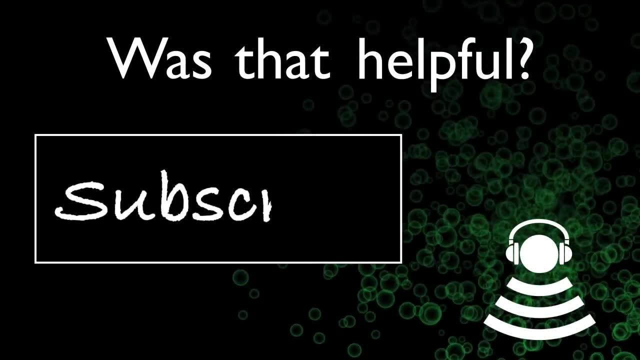 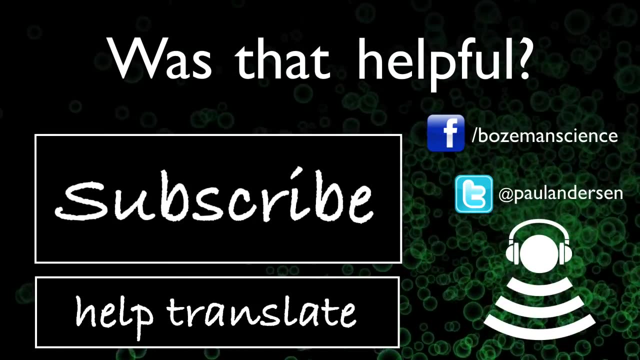 Remember, as we go up and to the right, we're going to increase electronegativity, based on Coulomb's law and the shell model, And I hope that was helpful. Thank you very much.